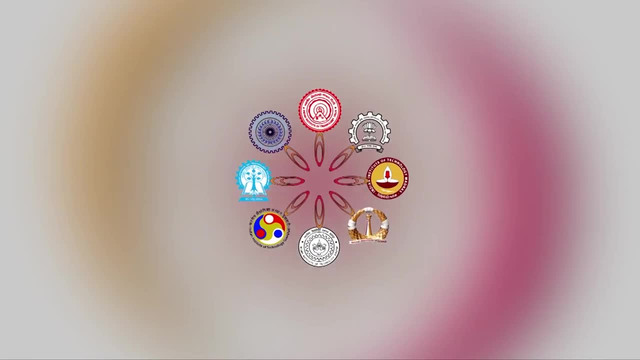 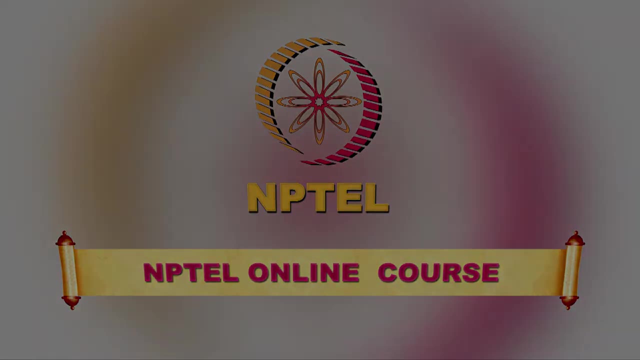 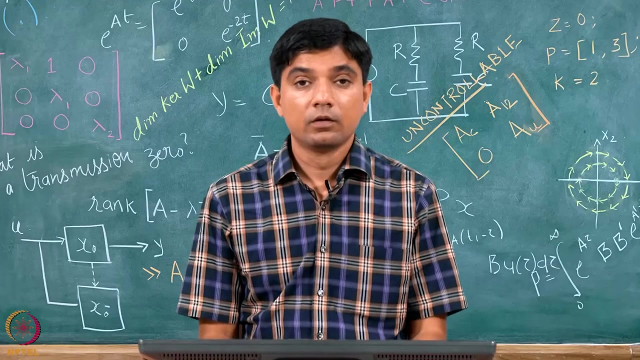 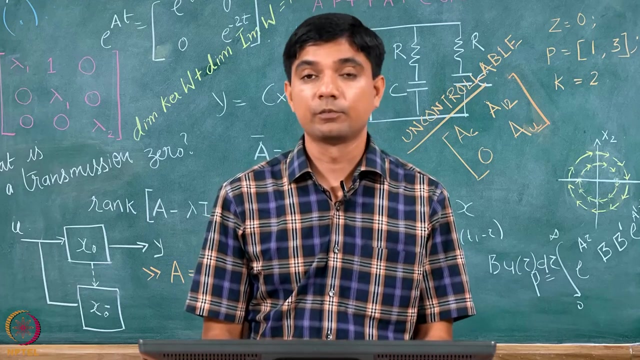 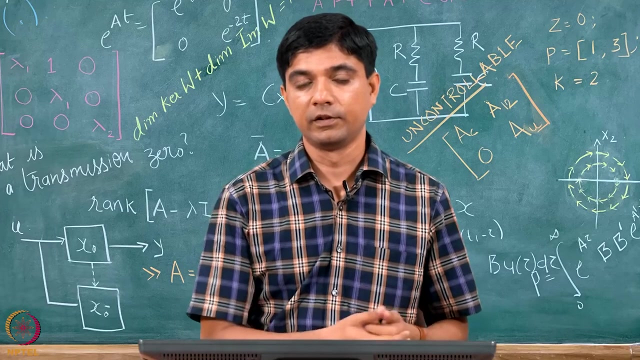 Hello everybody, my name is Ramkrishna. I am from the Department of Electrical Engineering, IIT, Madras. So welcome to the third module of the lecture series on Linear Systems Theory. So far in the previous- in week 2,, we have covered some basics of linear algebra, starting. 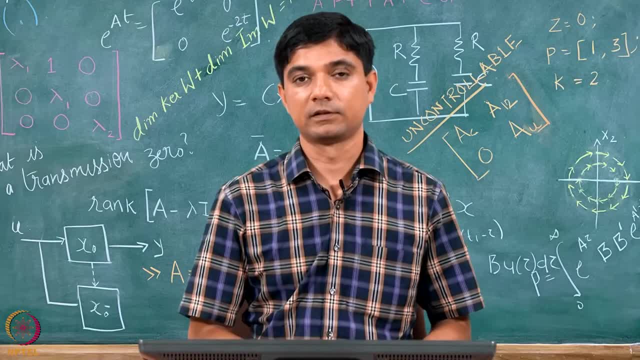 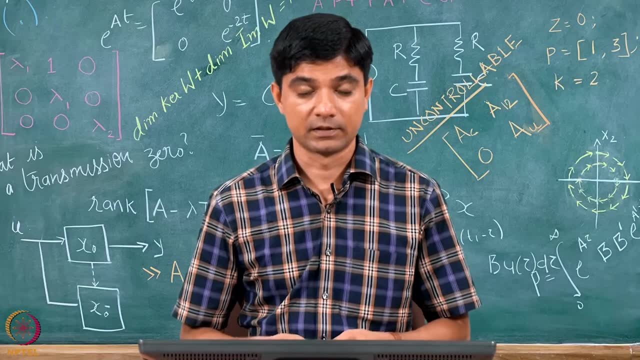 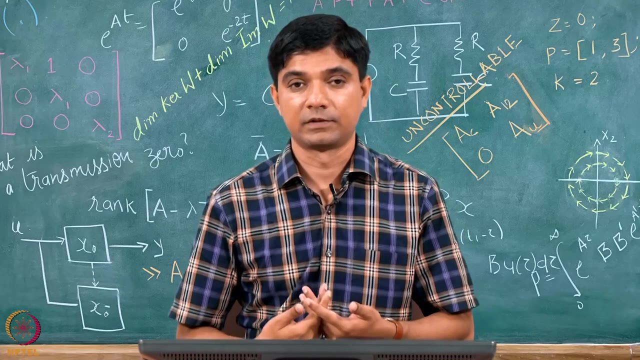 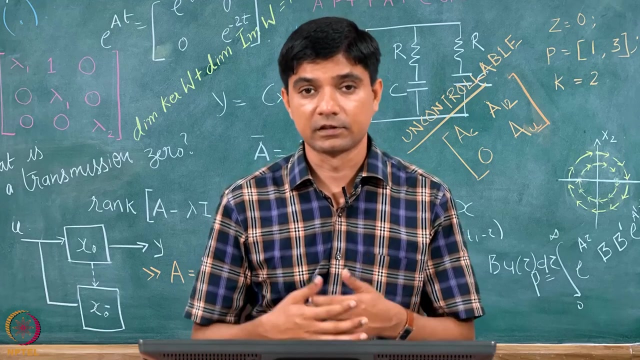 from vector spaces to normed vector spaces, to what is a linear transformation and how a linear transformation essentially has a matrix representations, And all this we need because we want some nicer tools to analyze systems at hand. you know which we write in the state space form. So we just continue our discussion on the 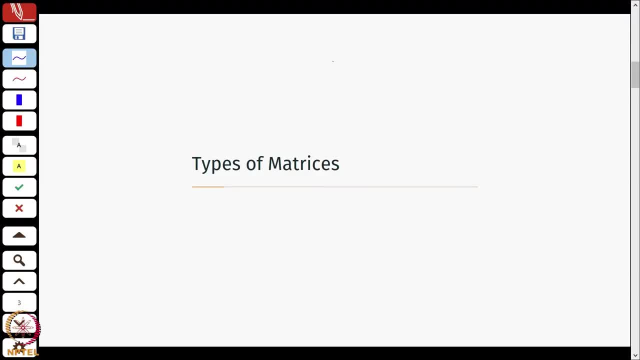 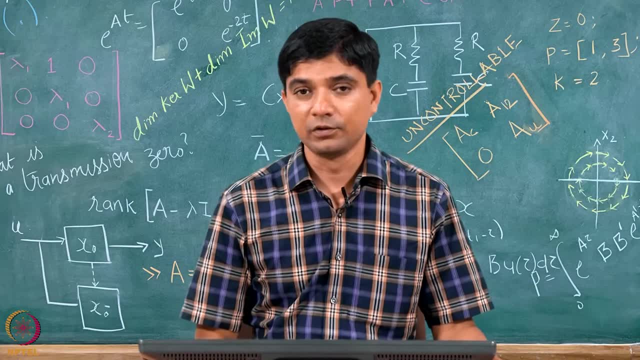 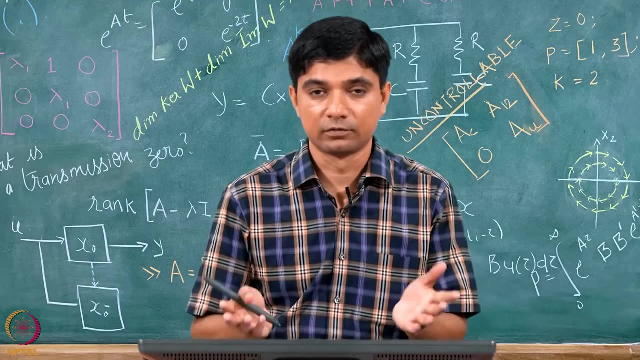 properties of matrices and vector spaces. First we just look at some very basic types of matrices. much of this would not be surprising to you. some of them might be even like intuitively clear. So we just run through those definitions just to maybe make the slides or the course. 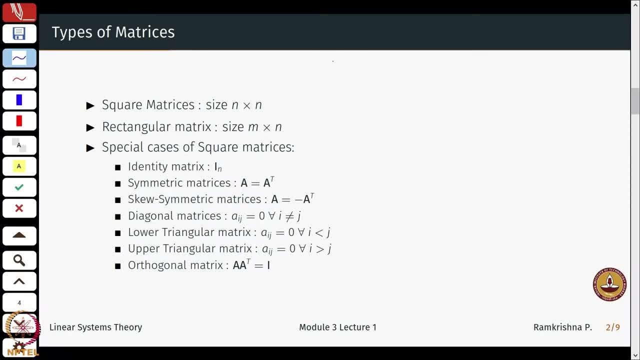 a bit self contained. So we have matrices where the number of columns and the rows are the same. rectangular matrix would be of a size m cross n, where m can be less than or even greater than n. So you can have matrix which are which has more number of rows and columns, and vice versa. So even 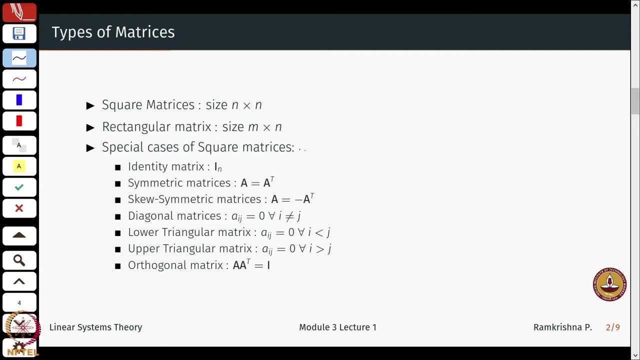 though much of our analysis would be restricted to square matrices and therefore we will spend a little more time on looking at that. So we have a couple of such properties of those. So first is the identity matrix. we will denote it as I n, which means it is like a n cross n. identity matrix, Sotypical I. 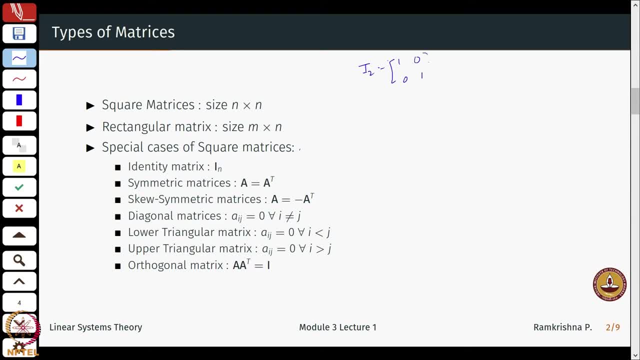 2 would look like 1, 0, 0, 1, and then we will just try to memorize this notation. Symmetric matrices, a will would be equal to A transpose, and I think we all know what the definition of transpose of a matrix is. 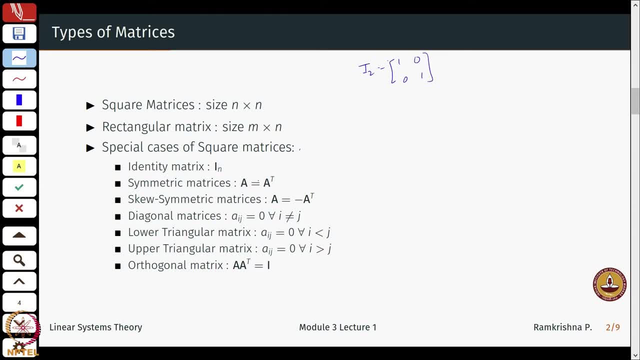 we have skew symmetric matrices where A is the negative of A transpose, say. a simple example would be something like: this is a skew symmetric matrix. You can just look at, just substitute and then and look at it in terms of each elements of the matrix. 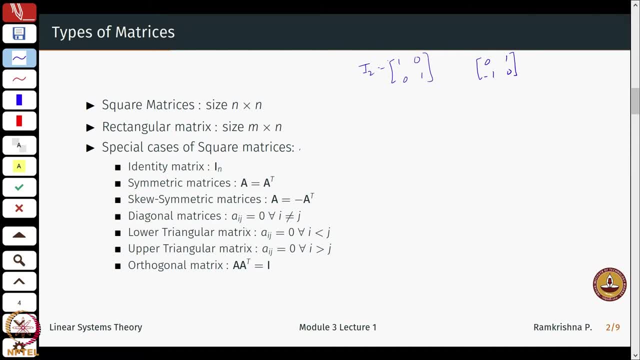 Diagonal matrices. where so the by definition it says A i j will be equal to 0 for all i, for all i not equal to j. So here A i j essentially is would represent the each of the element of a matrix. say, for example, if I take a 2 cross 2 matrix, this would be A 1- 1, A 1- 2,. 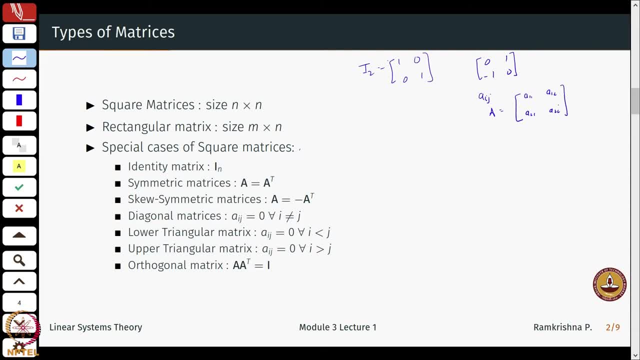 A 2 1, A 2- 2 and by the definition of diagonal A i, j would be equal to 0 whenever i is not equal to j. So this here, i is not equal to j, i is not equal to j and therefore A 1: 2. 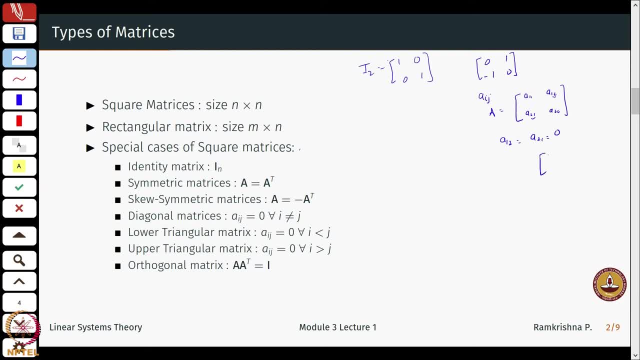 would be A, 2, 1 would be 0 and then the diagonal matrix would be 0. So it would just look like this. I am like very, very straight forward. it is nothing really to explain much here. Some more definitions of what is lower triangular matrix, again by: 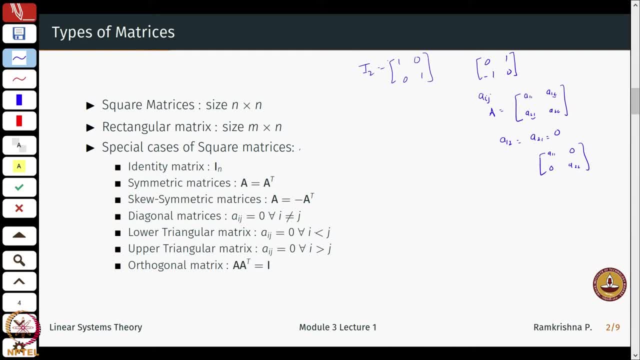 definition. it says A i j equal to 0 whenever i is less than j. If I just look at this, what are the cases when i is less than j? there is this one, So a matrix lower triangular would be something like this, Or, in general: 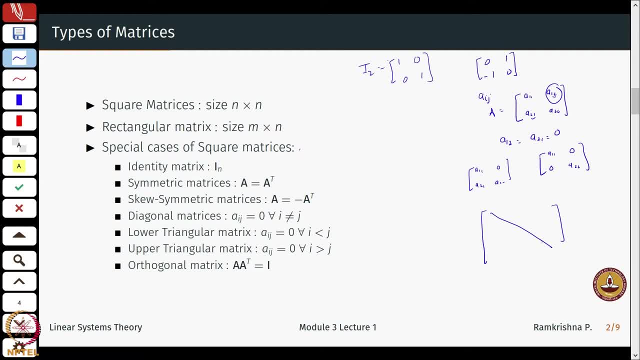 If I have a larger matrix, I have the diagonals here. So a lower triangular matrix would mean that all entries to the right of this diagonal- if you can call this right direction- is 0, or this is the actual definition. Similarly, in an upper triangular matrix, A, i, j would 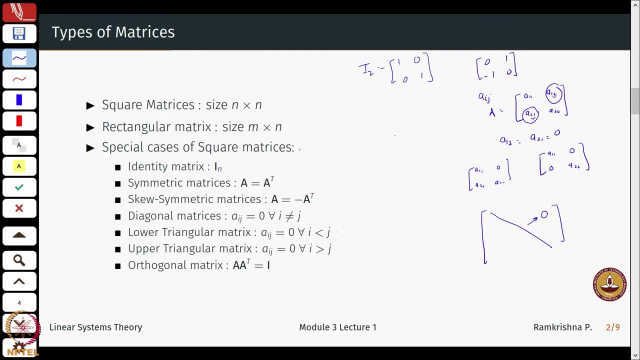 be 0 for all i greater than j. So this is the case when A 2- 1 would be equal to 0 and the upper triangular matrix would look something like this: A 1- 2.. So A 1- 2 is 0 here and A 2- 2, and we are not really worried about what is sitting on the 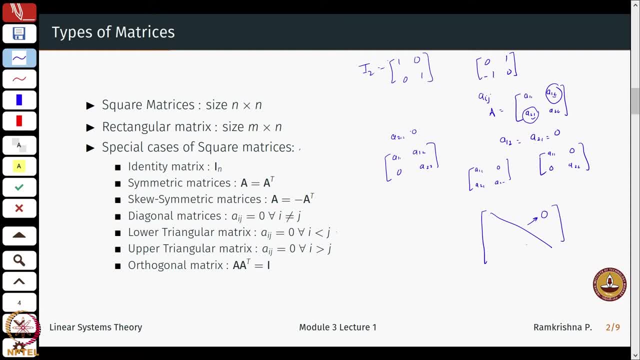 diagonal And in an upper triangular matrix you will have, all the entries to the left of the diagonal are 0. So this is lower triangular and this is the upper triangular. And of course, the last thing is an is that of an orthogonal matrix where A, A transpose. 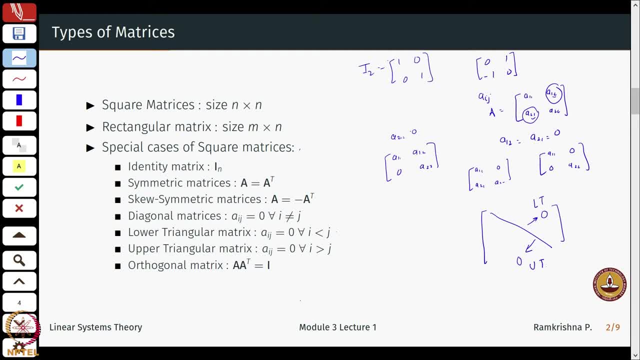 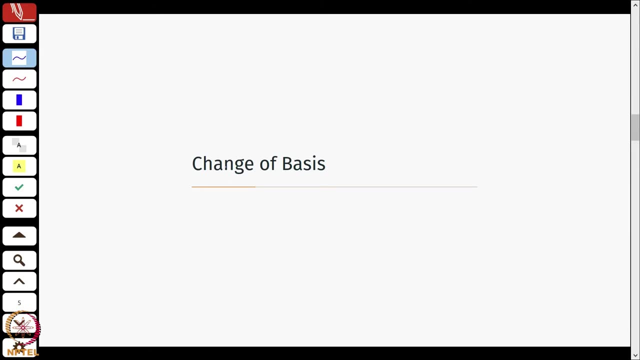 is the? is the identity of of appropriate dimensions. So whenever we just say identity, we will make sure that we are working with the appropriate dimensions. Specifically, when I need N, I will say I n is the N cross N identity matrix, something which is important And we will revisit this. 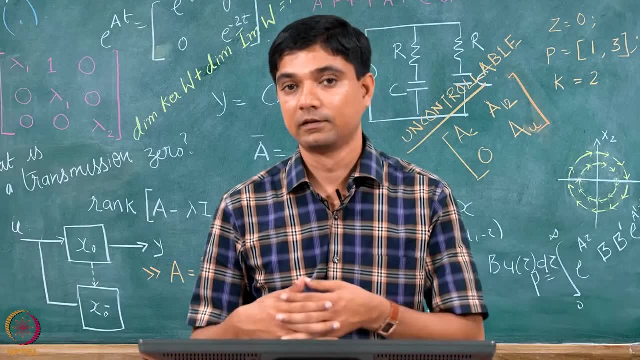 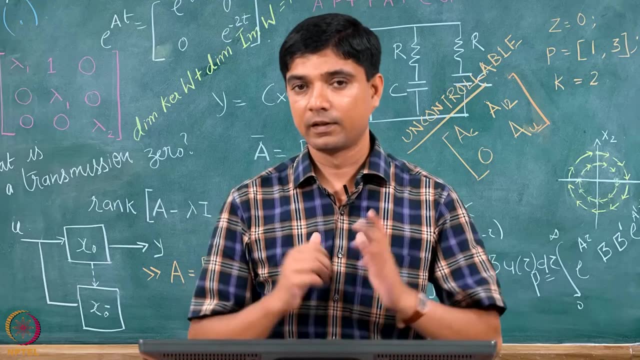 concept a lot of times in during the next few weeks of lectures. One is called the change of basis. If you remember a bit of a state space analysis. if you do not remember, does not matter, we will do it all over again. Change of basis. 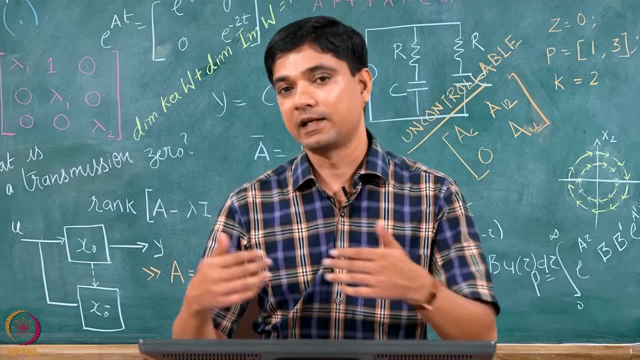 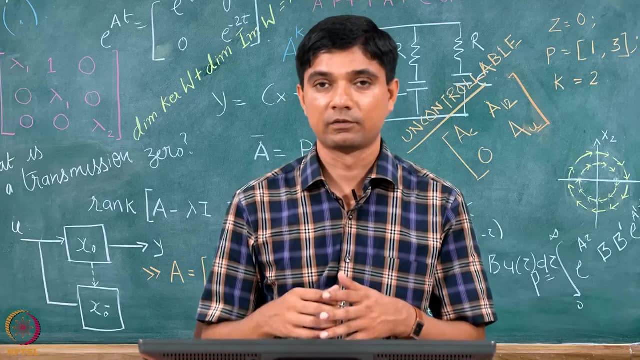 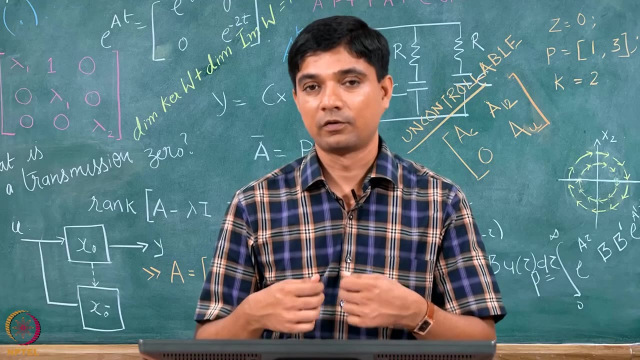 essentially means how do I change? or it is a direct implication on how do I change from a controllable canonical form to an observable form or a diagonal form or so on, or, given any state space representation, how do I go about deriving one of those canonical forms? 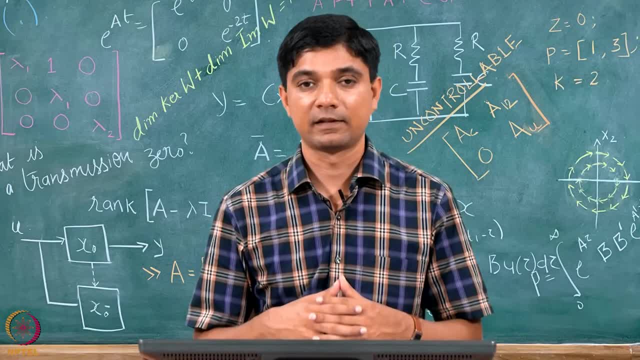 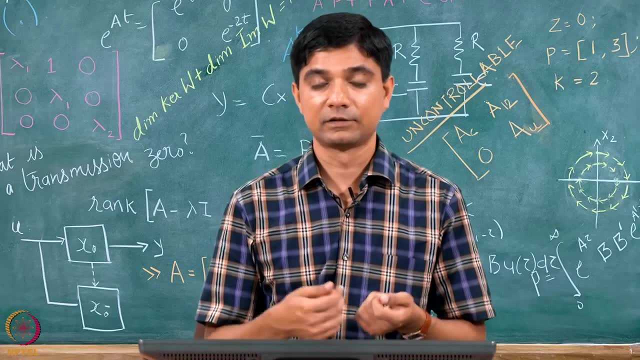 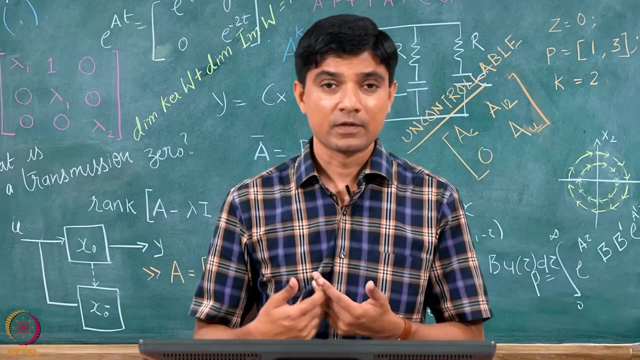 And the basis of that, or the mathematical tool for that is what we call as the change of basis. and what is basis? well, basis, if I look at the standard basis for two dimensional space, it was the 1, 0, 0, 1. and what we also did- a little example- is that, given a vector, 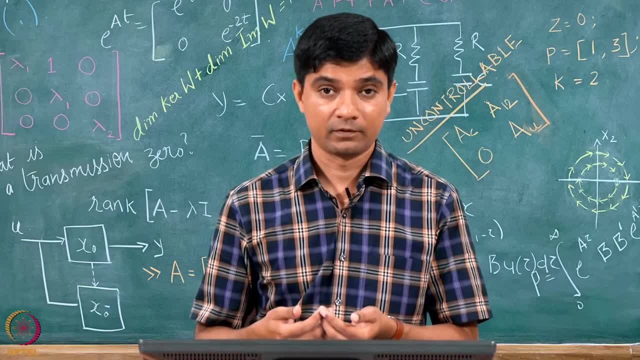 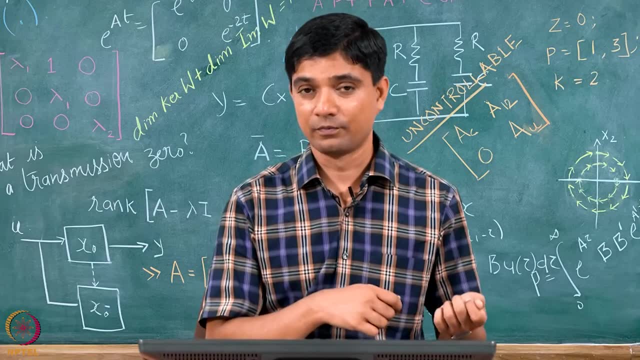 space R n. the basis may not be unique, right, And therefore we have to emphasize how. what is the thing that causes the change of basis? how do I go from a set of the standard basis to some other basis, right? So we will spend some time on that and also 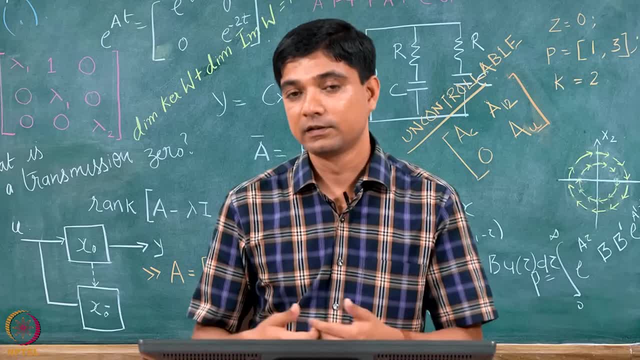 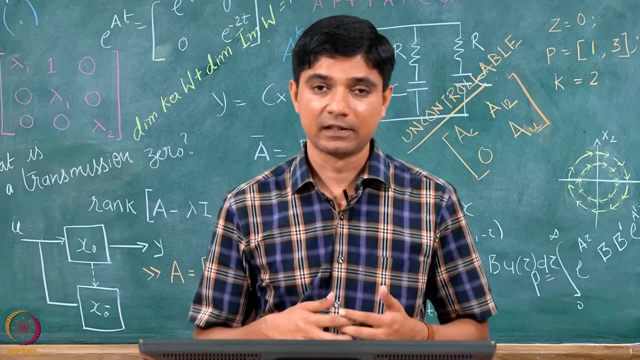 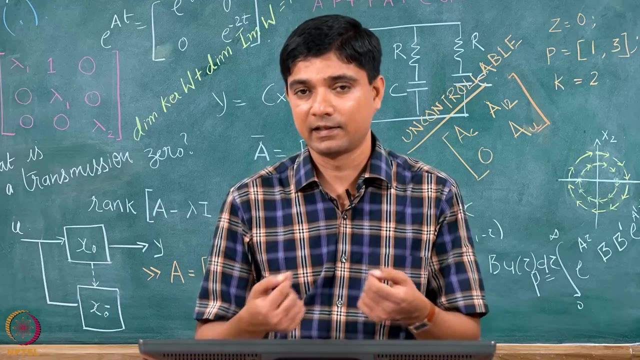 as. So as the lecture progresses today and further this week's contents, we will try and slowly relate to the state space representation of systems as and when needed, as and when, which is, it might be a little obvious, just to make a little link of the kind of tools that we 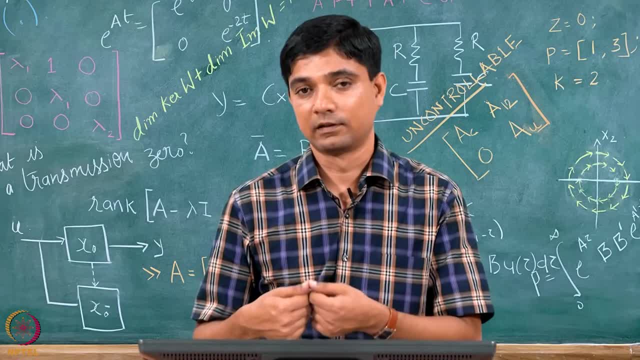 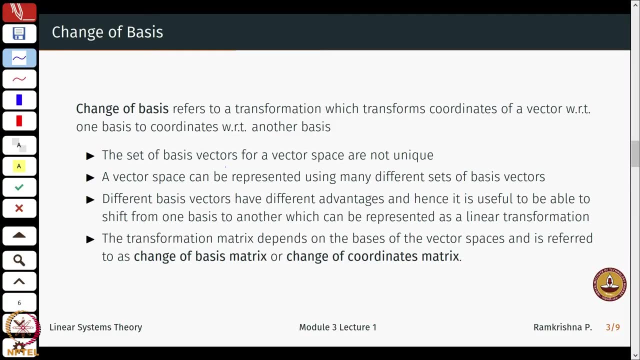 use here and how they are actually going to help us throughout the rest of the course. ok, So what is change? Change of basis: it refers to a transformation which transforms coordinates of a vector from one basis to another basis. ok, So transformation, I am talking of linear spaces and this transformation. 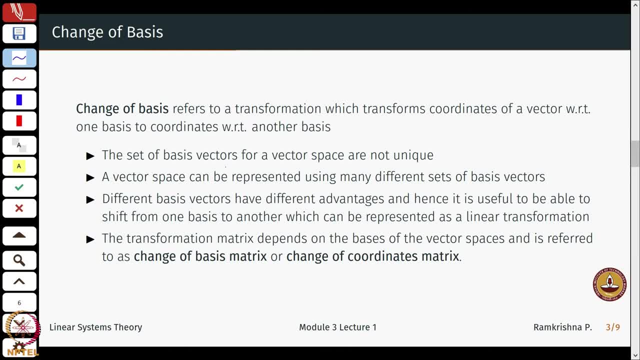 therefore, essentially will look like matrix. ok, And why can we do this, or why is this important, is because the set of basis vectors are not unique, and this actually is helps us a lot that the set of basis vectors is actually not unique. I mean throughout our coordinate geometry. we just look at the standard basis. 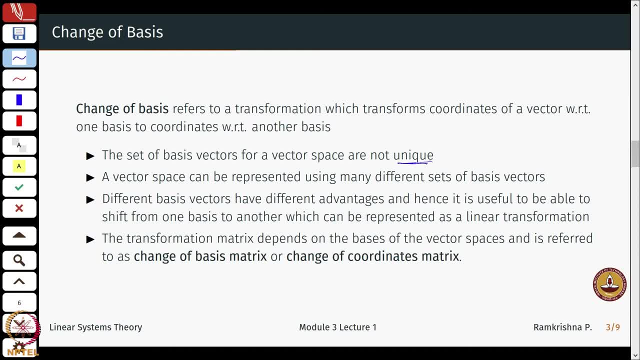 right and there. I am not sure if we ever encountered situations where we had to write in different basis, but here this is very important. ok, So the thing that we will exploit or try to analyze more is the property that a vector space can be represented using many different 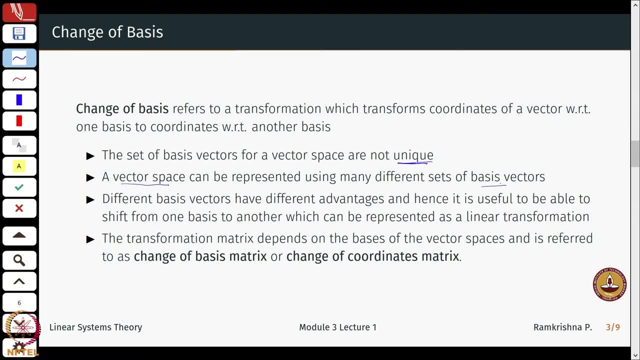 set of basis vectors. ok, As I said earlier, this Set of basis vectors have their own advantages, especially in the course. So this is not just very abstract thing that we are, that we are going to learn, but this is something which has direct implications on the control related concepts that we will do later in. 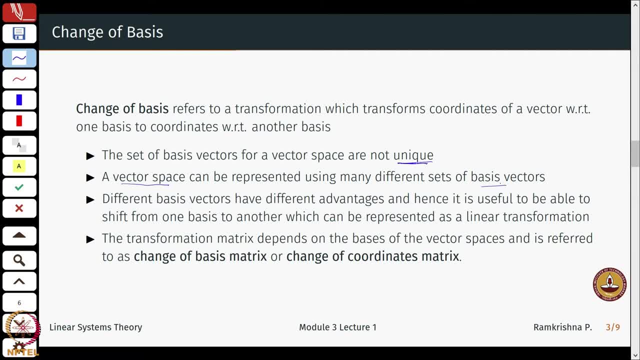 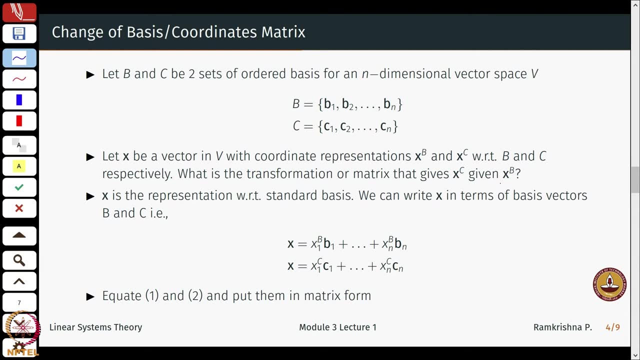 the course. ok, So how does what represents now the change of basis, or how do I go from one basis to other? It actually turns out to be a very, very simple exercise, So let us start with two different basis. So how do two basis relate? well, I just take two arbitrary basis. one of them could be: 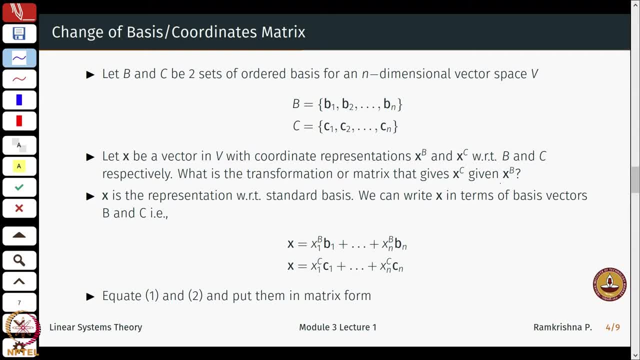 the standard basis for a, for a, for an, for a, R, n. it could be any of those right. So the transformation exists independent of what you do. So let me just take two basis, B and C, with their, you know their individual basis being from B 1 till B n, that the n vectors. 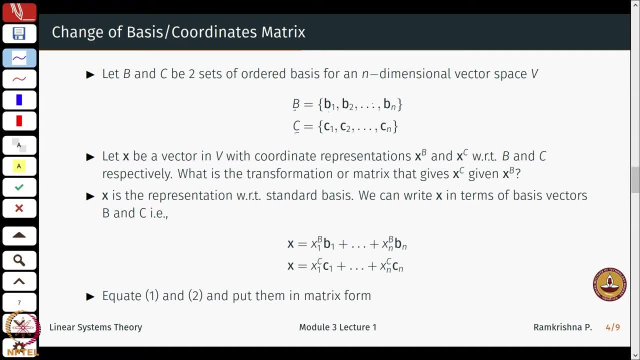 which represent Or which are set of ordered basis for this vector space V. here it is like: because you have n, this could be like R n. ok, So B 1 till B n. So this means that any vector in R n can be written as a linear combination of these vectors: B 1 till B n, The same vector. 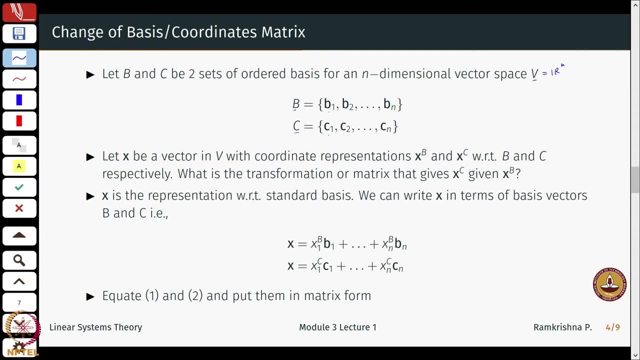 can also be written as a linear combination of this basis vector: C 1 till C n. and if you remember what we did for the, for the basis vectors, right? So we were talking of of linear dependence, linear independence, and B 1 to B n will form. 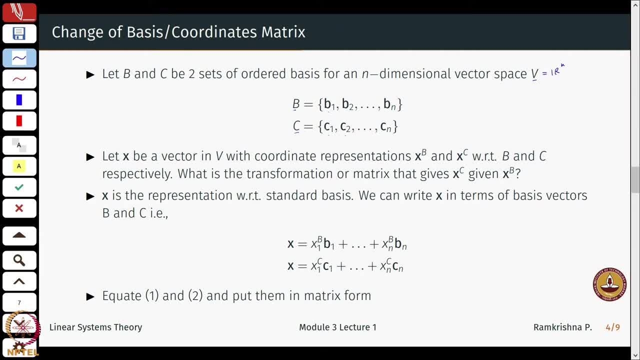 a set of basis if any vector can be written as a linear combination of of these vectors, ok, So let us start with X, Vector X with its own coordinate representations: x 1, x 2.. So So what is the coordinate representations? 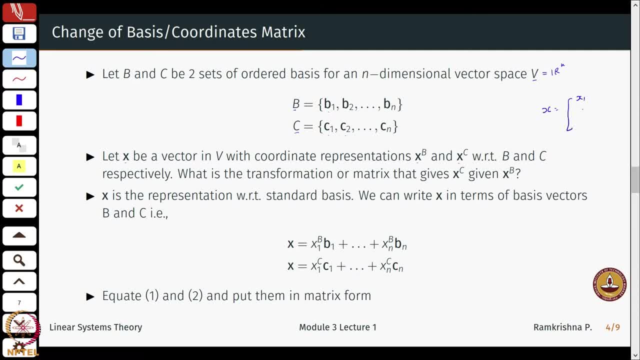 given x, I will have, if I can write this as x 1, x 2 all the way till x n. This, this is a coordinate representation of a vector, which can also equivalently be that I am writing this as x 1, say, the basis vector is b 1 till x n, b n, ok. 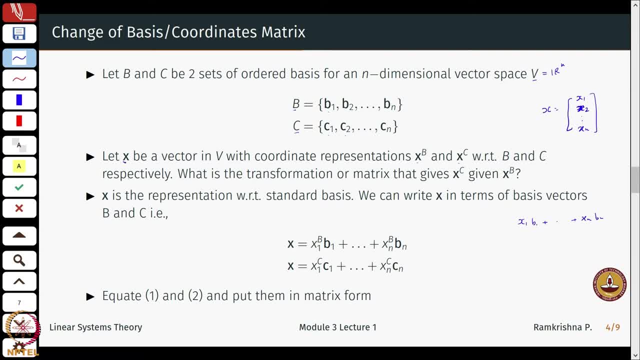 So let x be this coordinate vector, sorry, be a vector with coordinate representations x, b and x c, and the same vector can have different coordinate representations depending on what basis we choose. ok, What does that mean in when I write it on explicitly: So this vector. 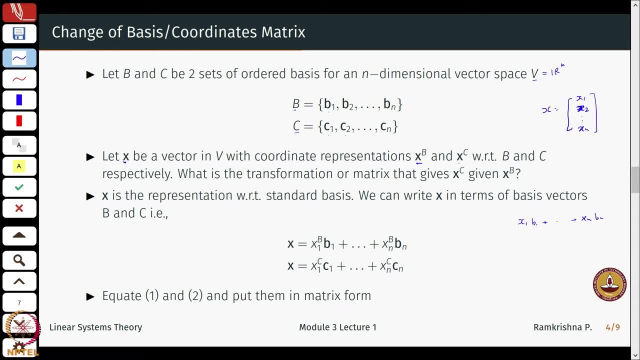 x with x b as a coordinate representation with respect to the basis. b can be written like this: right x 1 b, where x 1 b till x n b are the individual coordinates for this guy, x b similarly with x c. So this x can be written as x 1 b times b 1 till x n b times. 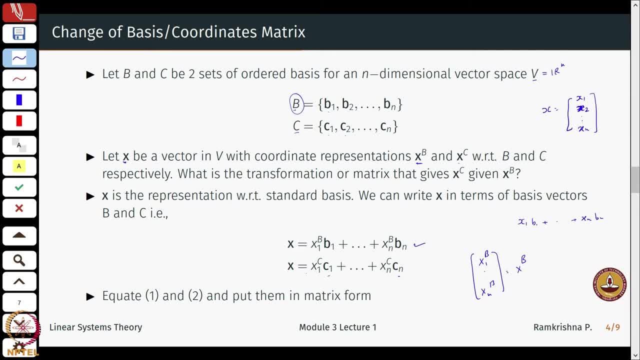 b n basis c can be written in this way where? ok. So what changes? since the basis change, the coordinates will also change. So I will have x c written as x 1 c all the way till x n c. ok, Now, these two are the same vectors. if I draw it on a sheet, I think they will. 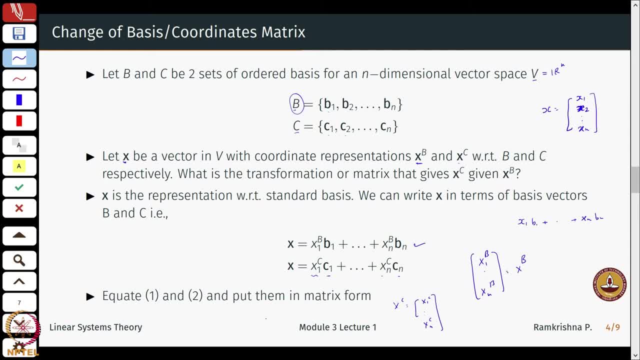 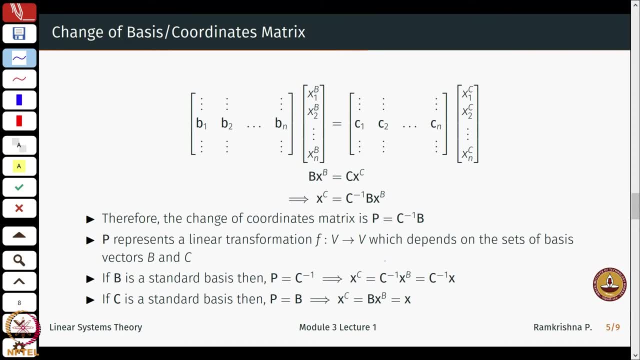 they will look the same. you can just do it. check by yourself that these two are essentially the same vectors. ok, So in matrix representation I can write this: b 1 times x 1, all the ways of something like this. ok, similarly with this one. ok, Now let me call this matrix. 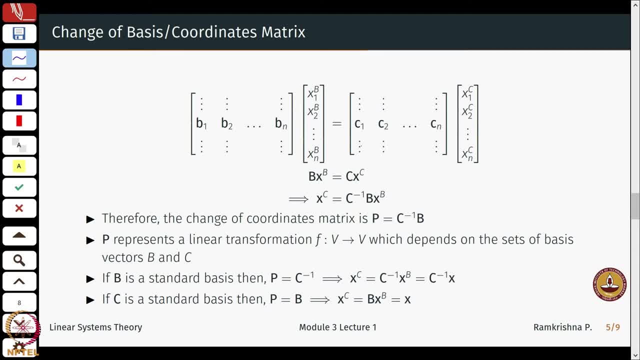 which I already called this, where this is b and this is c. So what I have here is b times x b. the vector x b is c times x, c, right in standard, if I just write it in terms of matrices. And ok, Now look at this matrix. it has n independent columns. similarly with this matrix. 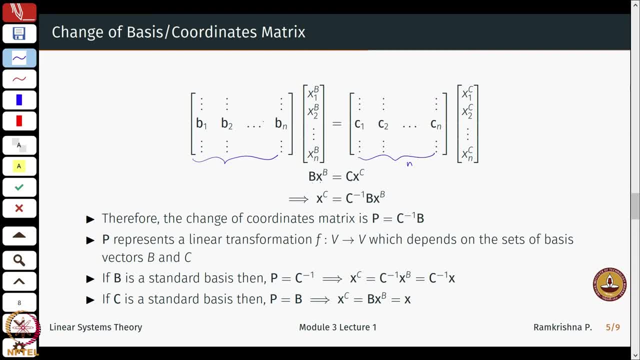 right. it has also n independent columns, because b 1 till b n are linearly independent. Why are they linearly independent? That comes from the definition of the basis. ok, So now, once these matrices are full rank, right, So this rank of this will be n the rank of this. 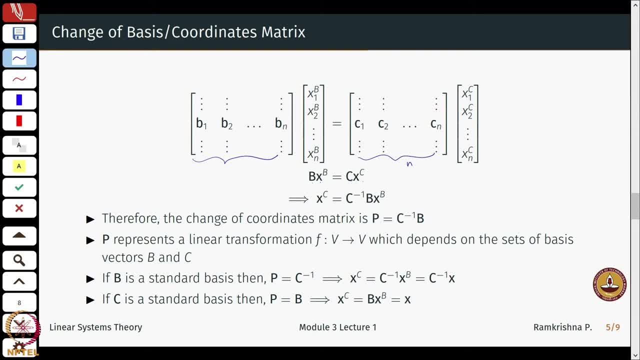 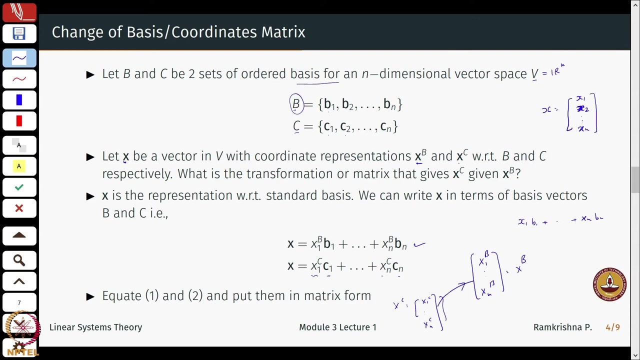 will also be n and I can interchange terms and write x c as c, inverse b times x b, or I can also do the reverse right. I can also write x b as b, inverse c, x c. So what does this answer me? So I have a vector, x c, this one right. So this things, what is the matrix that transforms? 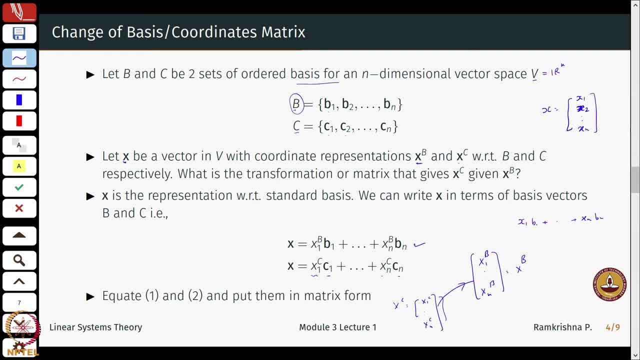 from x c to x b. So x c is written in this basis: c 1 till c n. x b is written in this basis: b 1 till b n. So what is the matrix or what is the transformation that takes me? 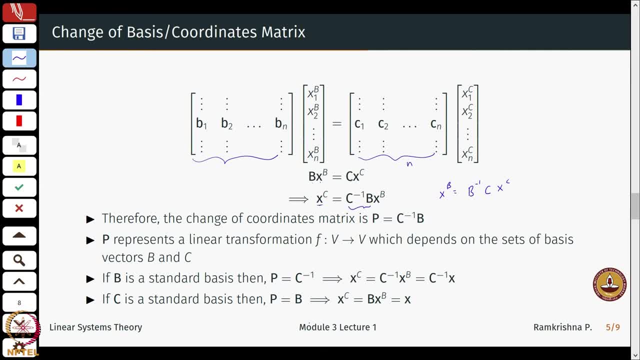 from one to the to other, that is simply this one. ok, So let me call this as p and this would simply be p inverse. and we all we know of why these are invertible matrices because of this n independent columns. ok, So what is this p? p represents a linear transformation, f from v to v, which depends 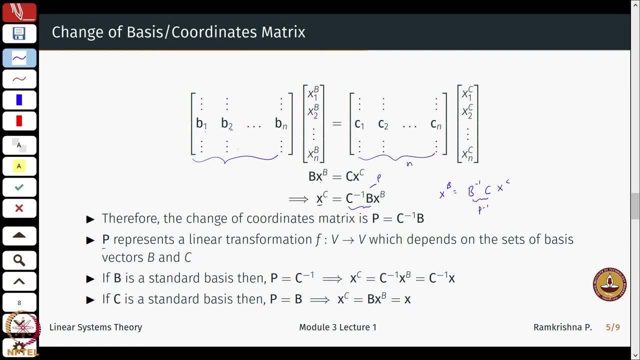 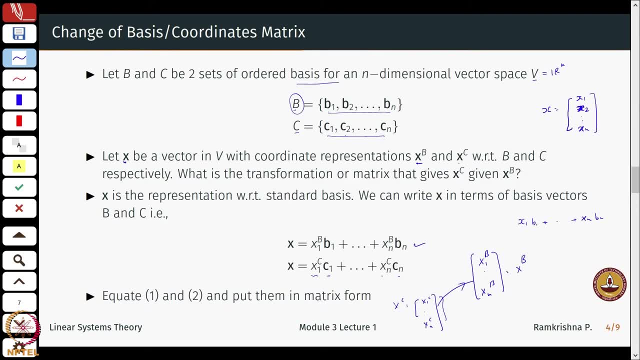 on the set of basis vectors p and c, right? So look at this, right? So these are the set of basis vectors for b. these are the set of basis vectors for c, right? So these two coordinates of the vectors x c and x b can be related by other basis vectors given. 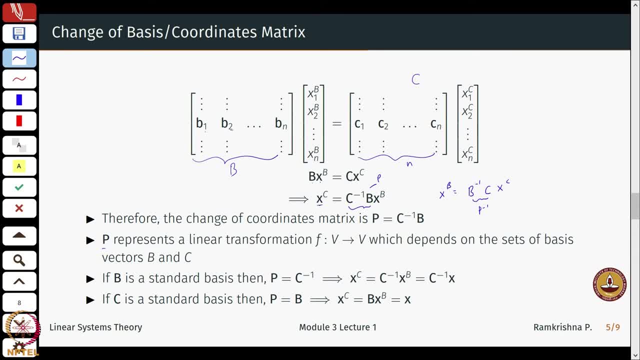 by this little relationship. It is a straight forward derivation, right. ok, If one of the one of them is a standard basis, say, let us say b is a standard basis and p is simply c inverse, because b is just the identity, right. So it will just be 1 0, 0, 0, 0, 1 0 0, all the. 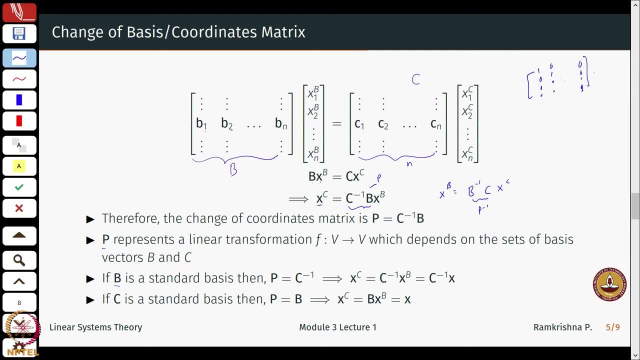 way till 0, 0, 0 and 1. this is a standard basis. let me call this as p. So, conversely, if c is a standard basis, then p equal to b and this is. this is like straight forward, then to derive. ok, So what we understood is how to go from one. 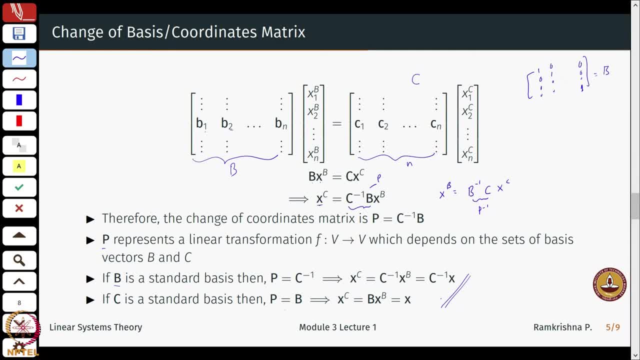 basis to To other basis, and this is this will be useful also- will also help to kind of memorize that such things actually happen. ok, And again, this transformation f from v to v is has a metric representation, p right. So this f is essentially has this metric representation. 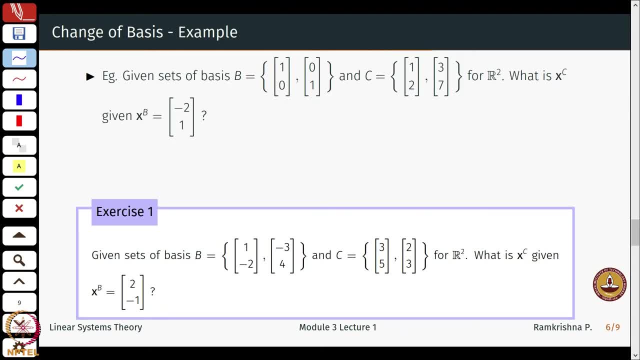 p. ok, Let us do a small example. this is pretty easy if you look at the basis b, this is the standard basis, as here and c is given, When, by this basis, you can check why these are basis. right, as a little exercise, these are actually linearly independent, and then so on. 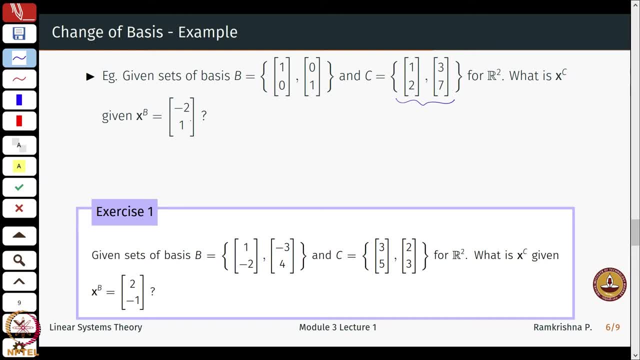 So what is x c when x b is minus 2 and 1? ok, So we just make use of this formula: x c is c inverse b times x b. Well, as it is, b is just the identity. So I am just looking. 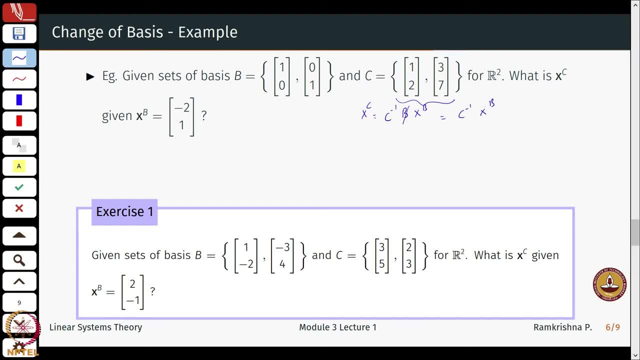 at c inverse times: x, b. Ok, C inverse can be computed easily to be 7, minus 3, minus 2, 1, and multiply this by a minus 2 and 1.. So this will be minus 14, minus 3 is minus 17 and this will be minus. 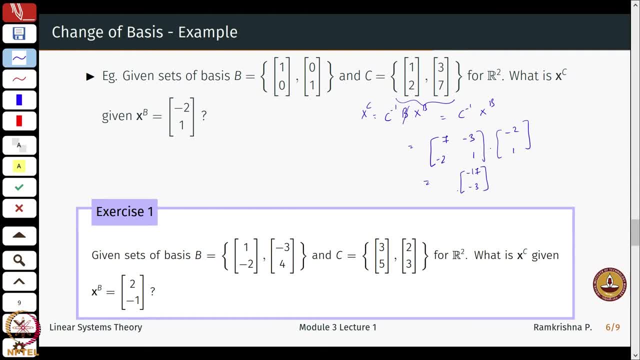 4 plus 1 is minus 3, ok, And this will be: 4 plus 1 is 5. ok, by just a very, very trivial exercise, And you can just draw these two vectors on a graph and check that they are. 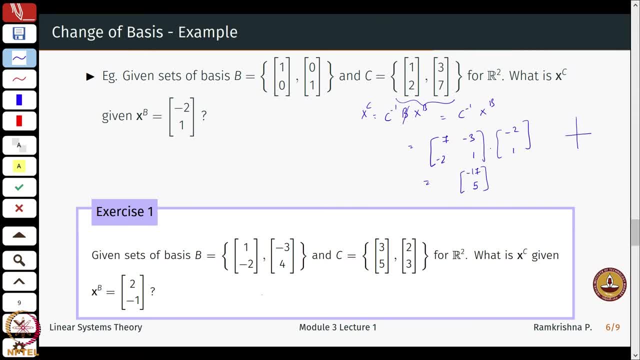 actually 0.0.0.0.. The 0.0.0.0. The same, and you can do a little more, not really difficult, but something which involves computing of one more inverse. So, instead of B being identity, I just give you a B matrix, which. 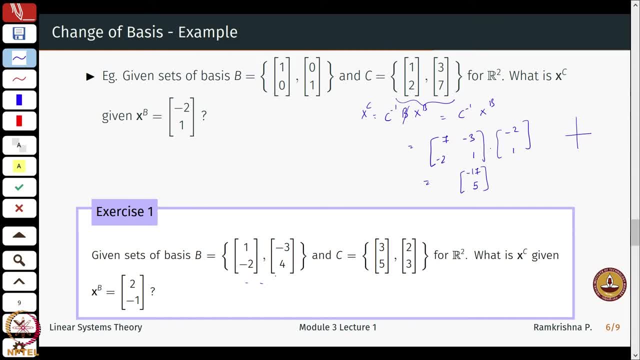 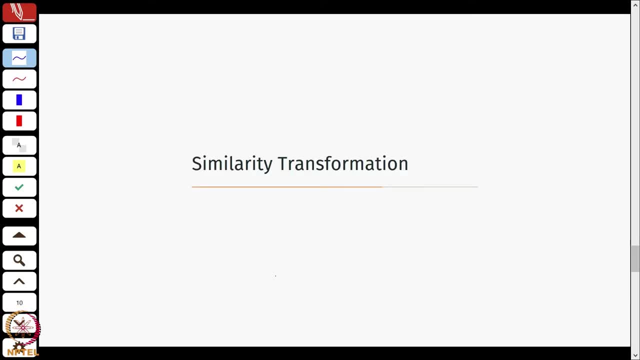 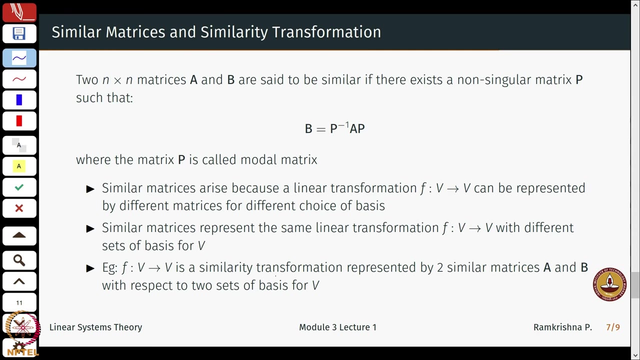 is like this. So there is nothing really special in this, in the slides or in this example. Let us do something which we would come across a lot of times, and this concept called the similarity transformation. So let us start with 2 square matrices, 2 n cross n matrices. 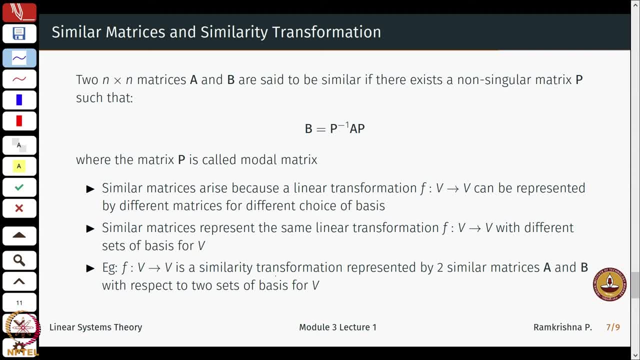 and by definition, and we will see why, what this definition means and where this possibly even comes from. So 2 matrix are said to be similar. if there exists a non singular, well, we need that to be invertible matrix P, such that B is P inverse A times B. 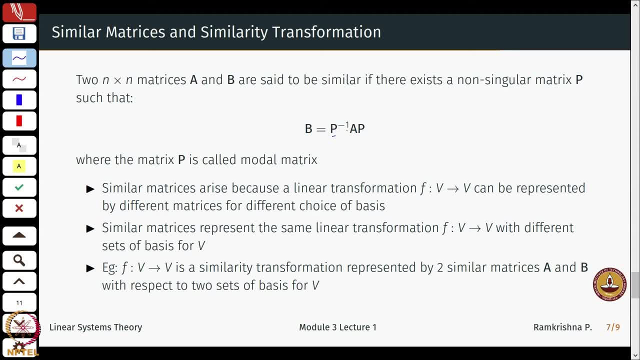 But P is called the modal matrix, where we will see how that comes from. ok, Now this arise because a linear transformation can be represented by different matrices for different choice of basis, as we saw here right. So we had 2 basis and you know, say, for example: 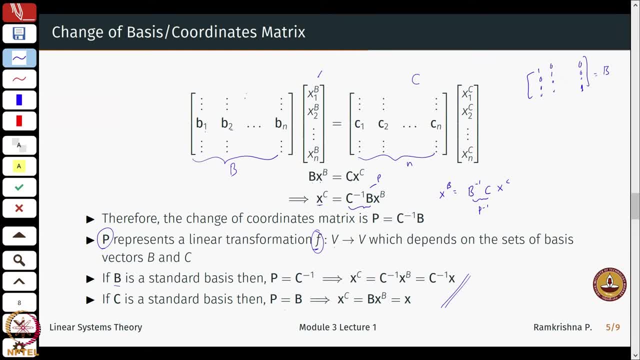 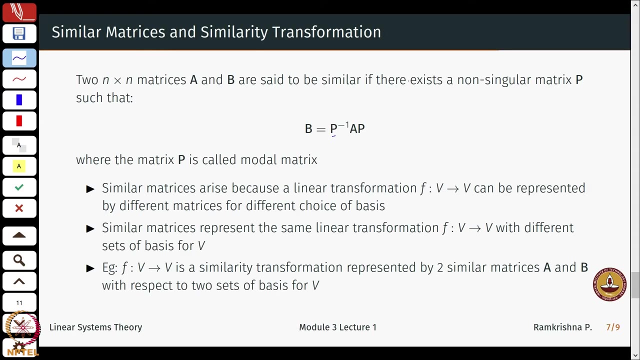 here. if these coordinates had a basis given by the matrix B, these coordinates or this vector has a, Had a set of basis vectors represented by this matrix C. So essentially, we are doing some kind of a special case of this one. So we ok, So this similar matrices represent: 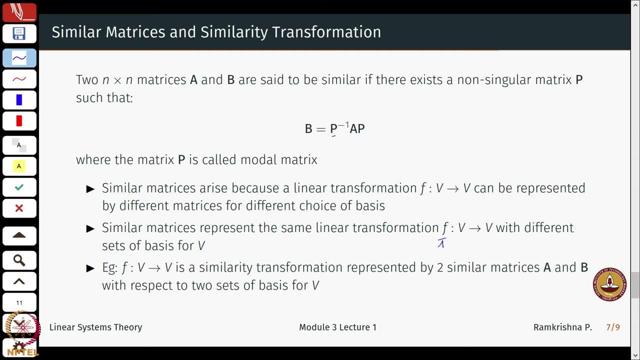 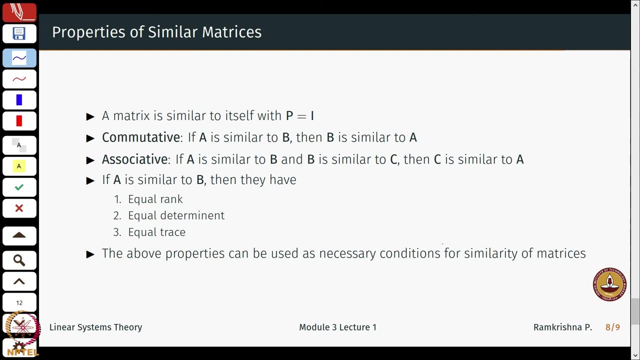 the same linear transformation. So whenever I say linear transformation, I am just talking here of some matrix A with different set of, With different set of basis B. ok, So what? how do we like derive this? a matrix is similar to itself, right? So what is the similarity transformation between P and P? So, and I 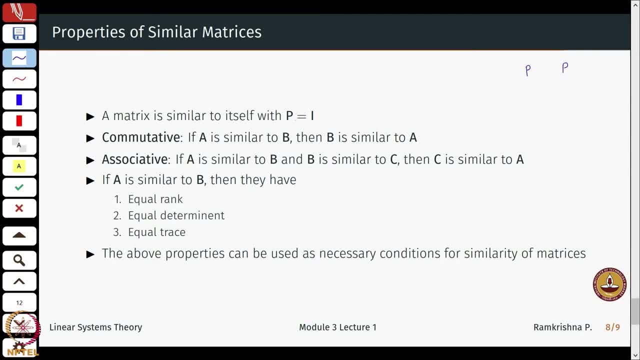 can say that this is just the identity, right, So it is P equal to a. So, ok, or take a matrix: A and A. what is P? the P turns out to be identity. this is trivial, ok. So second is, if A is, 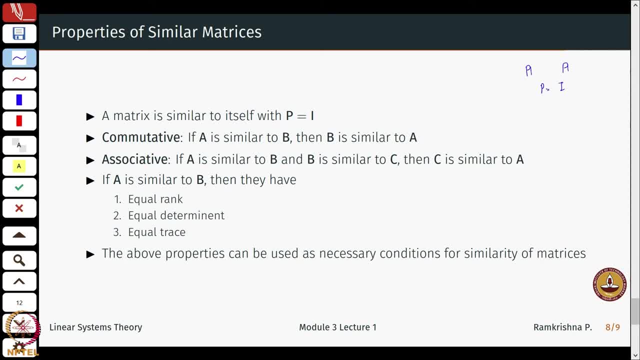 similar to A, then B is similar to A. So let us say that B equal to P inverse, A, P. right it is. you can even write A as now: P, B, P inverse. if I just want to write, I will just call this P inverse to be Q, and then I can write a new relation like this: Q inverse, B times Q. ok. 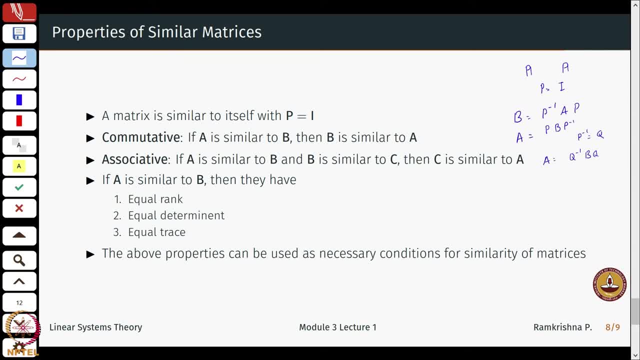 Then all those properties of associativity. if A is similar to B, So then you can write it as P, inverse B times Q. ok, So this is: A is similar to B, B is similar to C, then A and C are also similar. ok, So A is similar. 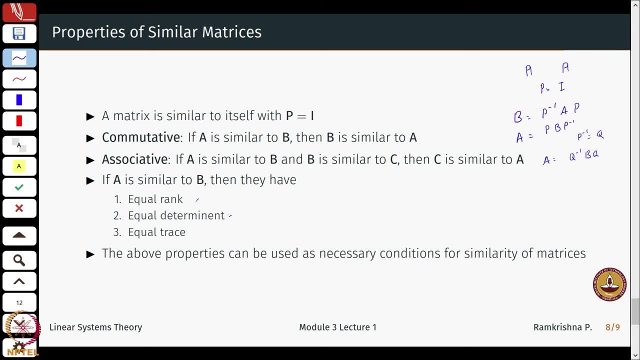 to B, then they have equal rank, of course, they have equal determinant. they also have equal traces, right? So ok, So we just do some things here. also why this is important. first, from the control point of view. So most of our, of our examples- 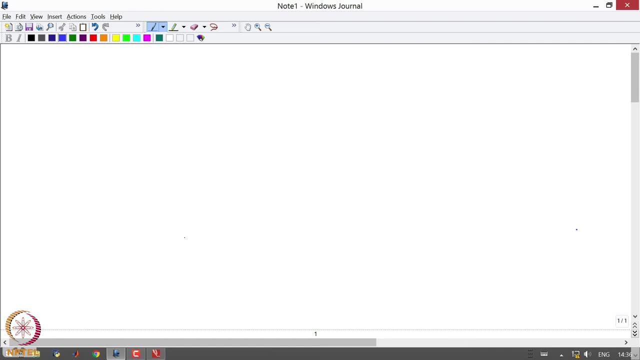 would look like this. So if I just say I have a system, x dot t is A x t the standard state space representation that we will substantiate a little more later. ok, Now suppose I were to write this in some other. these are all coordinate representations. 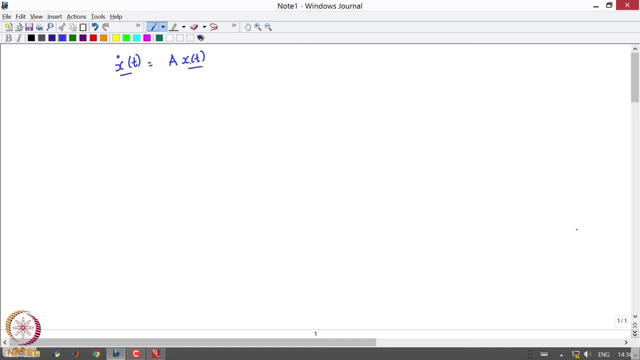 right x, dot, t, which are the states. these are essentially coordinate representations. where belongs to certain, say n dimensional space? ok, Now let me just call something that x equal to P times z. ok, So this is. omit the arguments in time. So this is t, this is t. 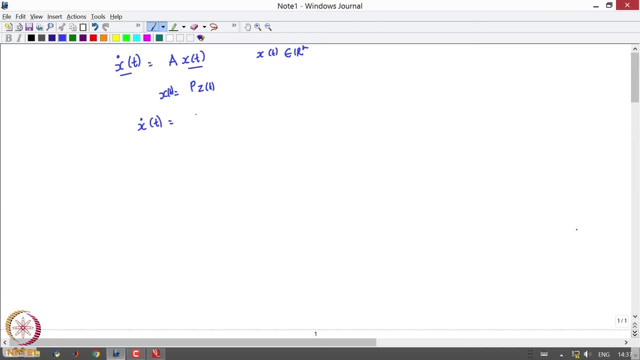 then x dot of t is P z dot of t. ok, Now what is x dot? x dot is A. I would also like. Well, let us think about that word x t, I would also. first I will- I will probably make some examples with P z dot of t. So let us think about some of those previous. machines. I would like to give some examples of with that. So, in what case it may be, x dot. x dot is A ningo P. ningo survive is A ningo d Phillips mRNA gradient voucher. RNA Yo-Jo성이 is an neural network, so this one may km if P. 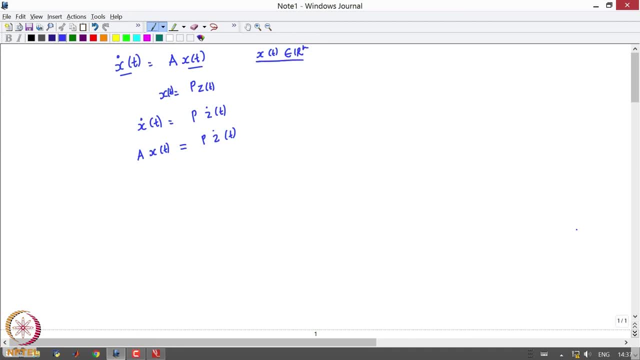 svi z ok k因 k x t equal to P, z dot of t. So now what I want to say, say, given my system dynamics in x, how would they look in z ok? So z dot and this, this is always an invertible. 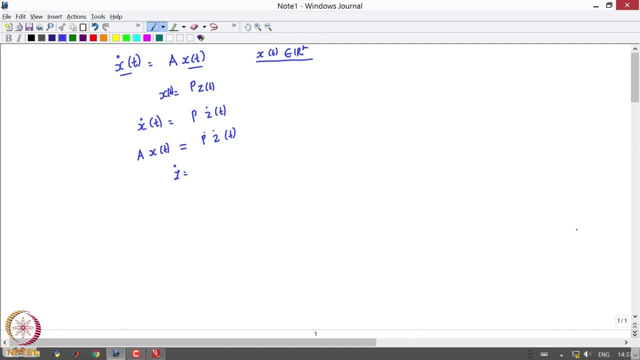 transformation. that is what that was in a the condition. So this z dot or P times z z dot is A x t or p times z dot is A. what is x in terms of p. So I will get A p z of t, or in other words, z dot of t is p inverse A p z of t. So this is my similarity transformation. 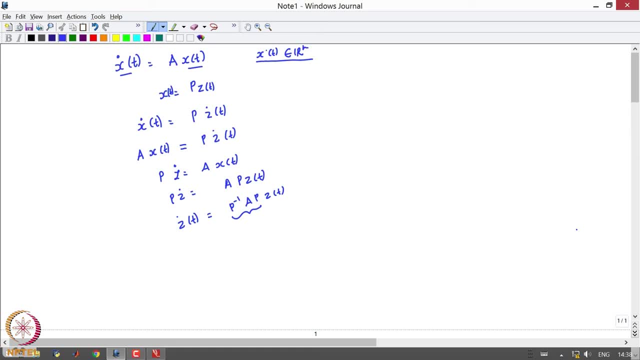 right which transforms my dynamics in certain given coordinates x to some other coordinates z. ok, Now, all properties, if we, if you remember vaguely of stability, were all related to the sorry, to the matrix. A right, So say, for example. so here I just said that, well, these are, these have equal rank, equal determinant, equal trace. 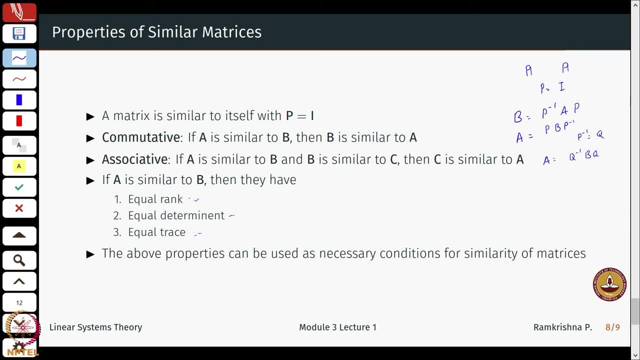 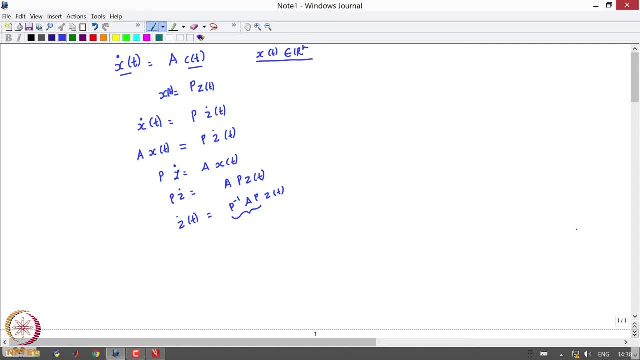 ok, maybe one of this would be easy, though equal rank is like easy to find out. So a very important concept I would always look at is: what is the implication on stability? and, if you remember, stability had something to do with eigenvalues or the basic properties. 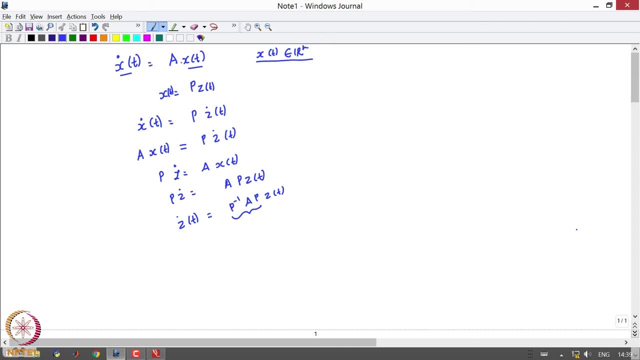 of the matrix right, even if I look at, in terms of my characteristic equation, the poles and so on. So how do the poles of the system relate in x to the poles of the system in z? ok, So let us, let us quickly do this right. So, 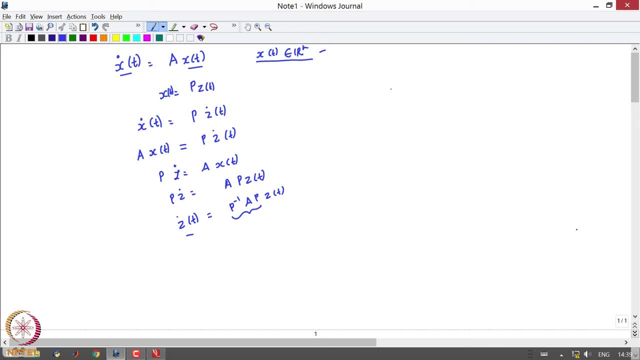 how do I? how do I find those? So I have lambda i minus p. inverse A. p is the determinant of this is my characteristic equation in z coordinates. ok, Now this will give me a set of eigenvalues, and I were to if I were to look at. So what I want to establish is the eigenvalues which come from this matrix. 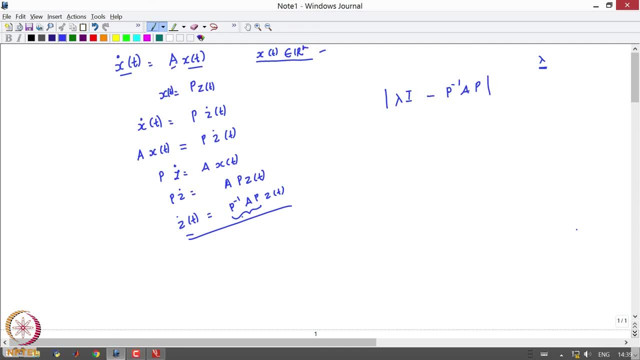 p inverse A p and how they relate, So how they relate to the originals, so to speak. A matrix. ok, I can write this then as p inverse lambda p, p inverse A p. We can do this is equal to p inverse. So inside I will. 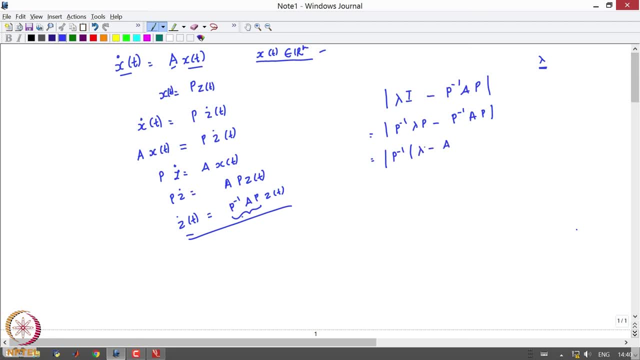 have lambda minus A. so just to make it consistent, Ok, Ok is put: lambda I minus A times P. ok, Now this is equal to P inverse: lambda I minus A times P, and this is lambda I minus A right. So the solution to the characteristic equation: 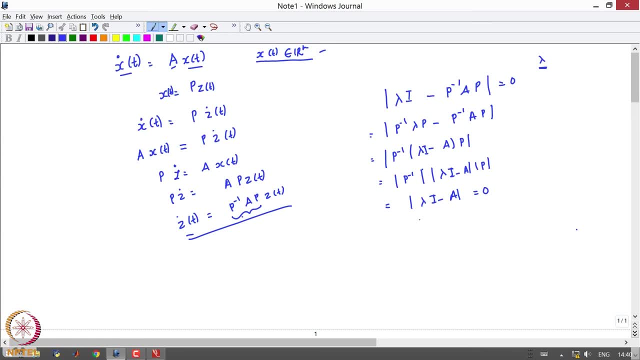 would just be to equate this to 0.. So if I equate this to 0, it is as good as equating lambda. I minus A to 0, and therefore the eigenvalues of the matrix A are the same as the eigenvalues. 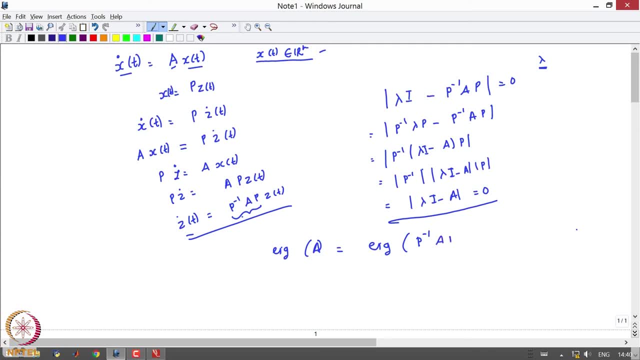 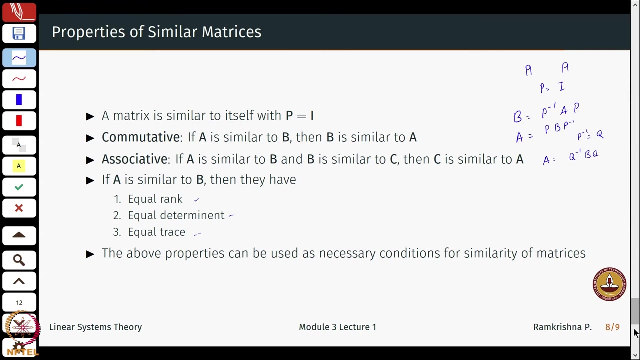 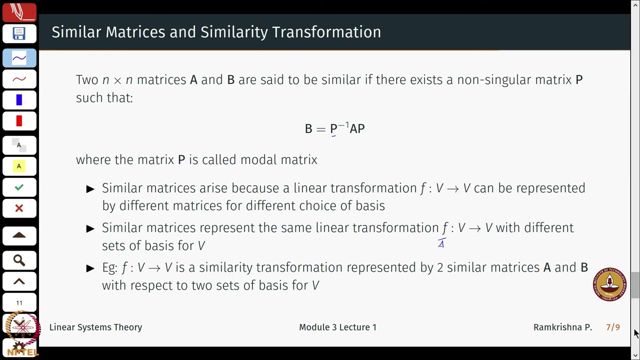 of P inverse A P, So much of the properties remain invariant right. I mean this is kind of intuitive also why these properties should remain invariant right, ok, So Now what does similarity transformation or how do this relate directly to a change of basis right are there? is there a nice interpretation of this, of this P inverse A times P? ok, So, 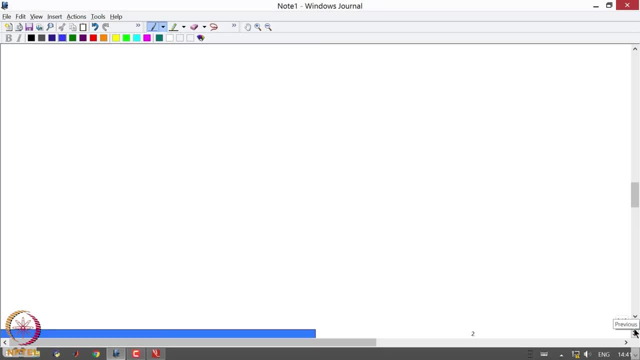 let us do a little scenario here, right? So I let me take a space- x could be of whatever dimension- and say it has the coordinates x, c, with b 1 till b n being its basis vectors. the same x has another coordinate representation. 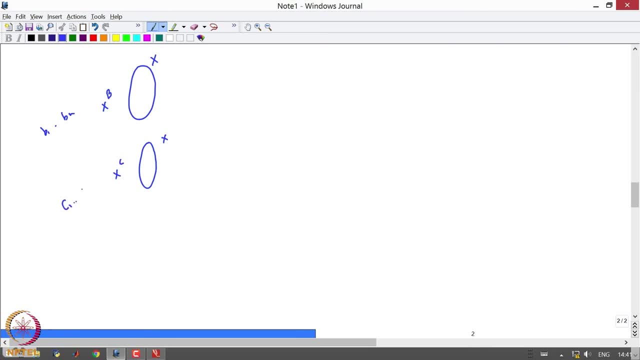 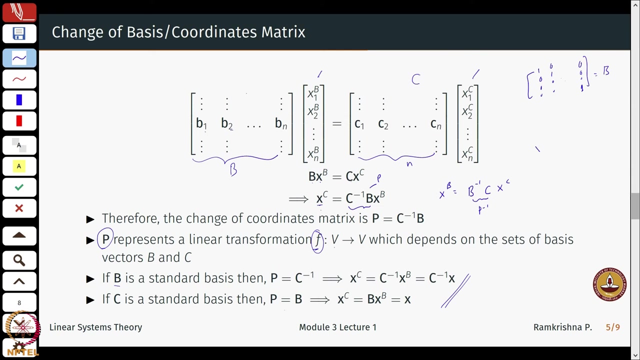 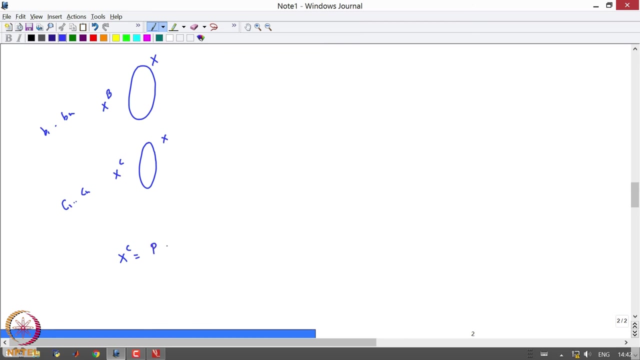 x c with c 1, c being c 1 till c, n being its basis vectors. ok, So what we saw is that. So if I, if I just were to rewrite this formula here- that x c is P times x b, ok, let us rewrite that here- that x c is P times x b. So it would mean that: 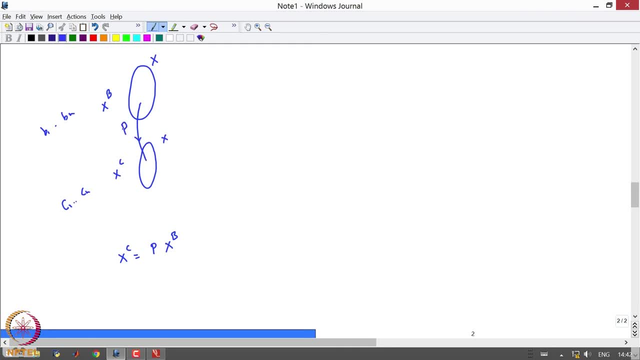 this P is a transformation which goes this way. this side, not this way, is correct, So ok. So P times x b will be x c, right, ok? Now assume also that I have another space, say y ok, which could be of a different dimension, say and has its some vector representation. 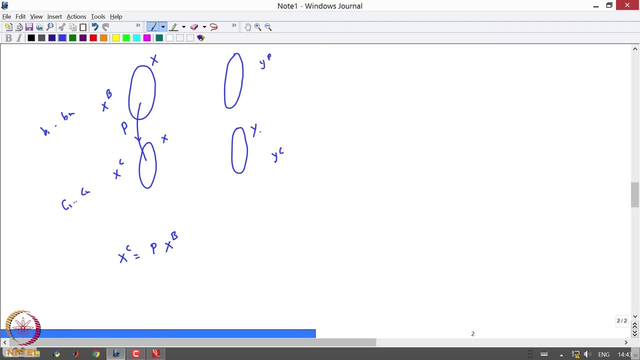 here as y c, some vector representation here as y b with its own set of basis. right, whatever they could be, you can just write whatever notations you want for that side. ok, Now We know. say, suppose there exist some transformation which goes, takes from, takes me from x, 2, y, and let me call that transformation to be: 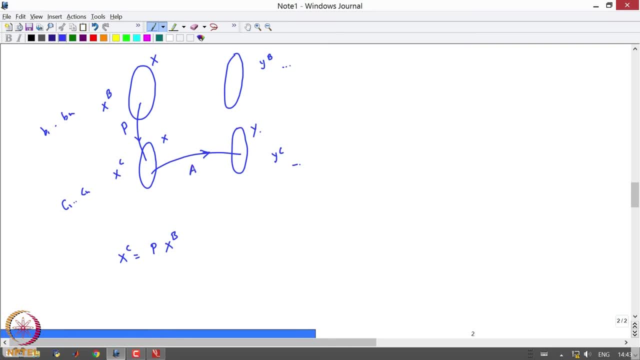 say some a. ok, This transformation should also exist here, right? So this, both this spaces are y, this is x, this is x and this x. the x on the on, on the top, has some basis representation: b 1 till b n- ok. 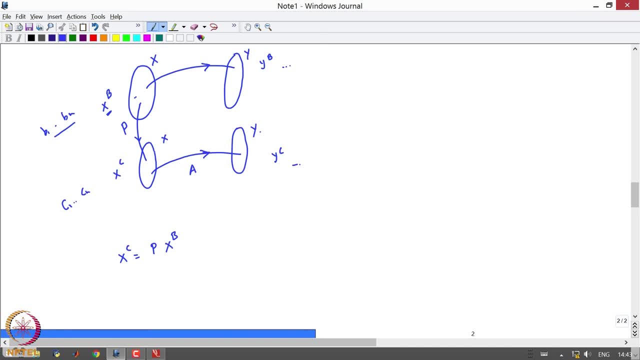 b, m with a certain vector, x, b. Similarly, over here the x on the bottom has vector representation x, c, with some basis: vector c, 1 till c, n. ok, Now, if I just look at A as a transformation from this x to y, maybe over here, right with this under this basis. So we always define. 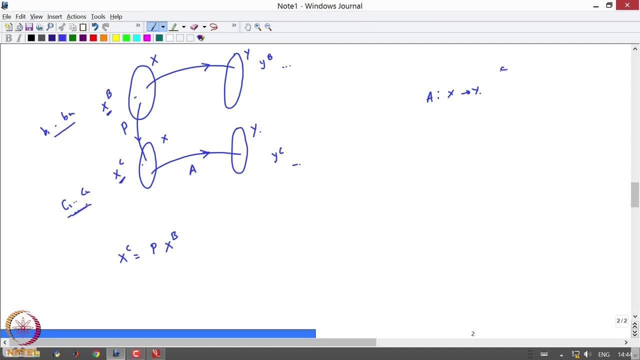 the transformation with basis. So let me call this. you just associate it to c, So it will not notationally correct, but let us see how. So this is how it looks like, or maybe I will just call it say: A, c. ok, There also exists a similar transformation from: 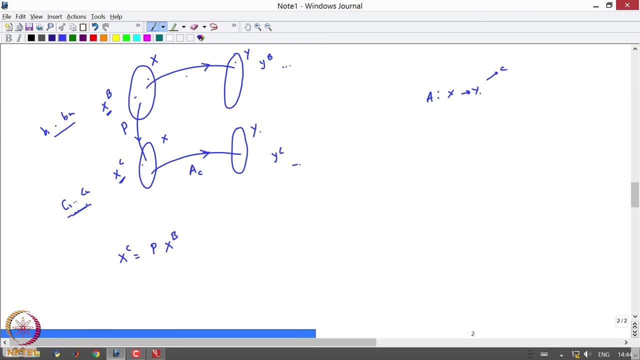 x to y under this basis. So let me call this A- b. So the question is: how does A c relate to A c? Ok, ok, now I know this. I can also define now a transformation which goes from y, b to y. 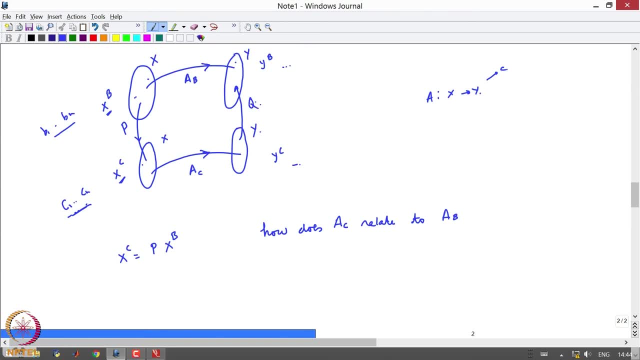 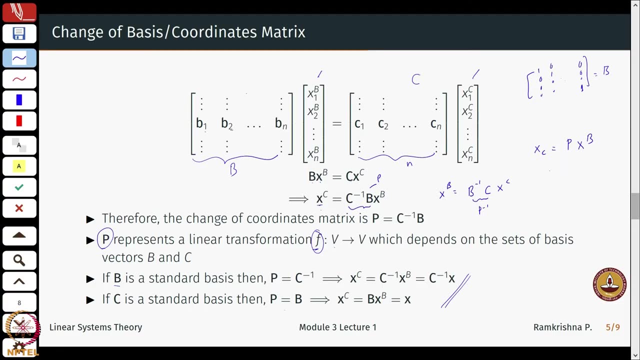 c via some matrix q, right? I mean I can just do whatever. I can even define this way, right, because this I was just So. if I can write x c in terms of x b, I can also write x b in terms of x c. sorry, x c here, not c here, whatever is. those is rotation, right Now. 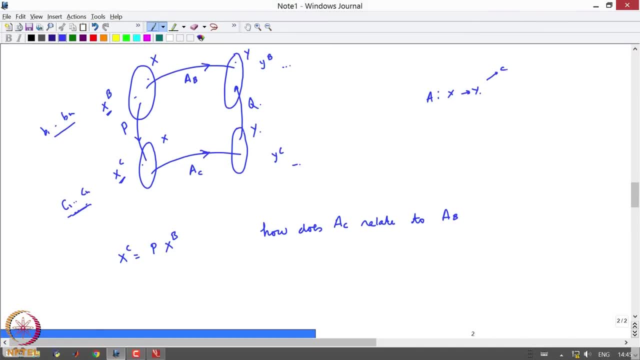 here is the, the term. So you see, if you define Yes here, so here is x, B is actually yellow that You can define it the term H of QB. So So I can just go from here till here. Now look at this carefully, So I can always write. 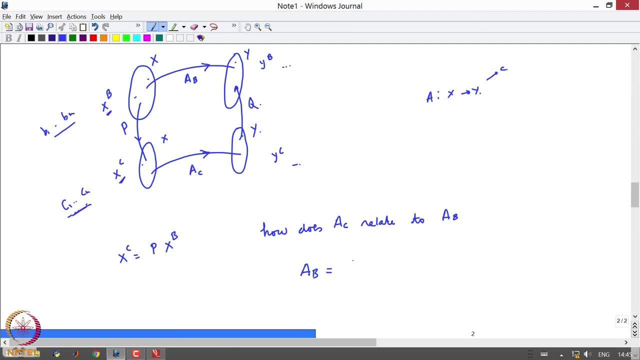 A B as P A C times Q, right. So this is a transformation which takes me from this basis till this basis, and it is the same of me going from this to this via A B is the same as me going via this route. So I take: go from here till here, then jump from here to here and 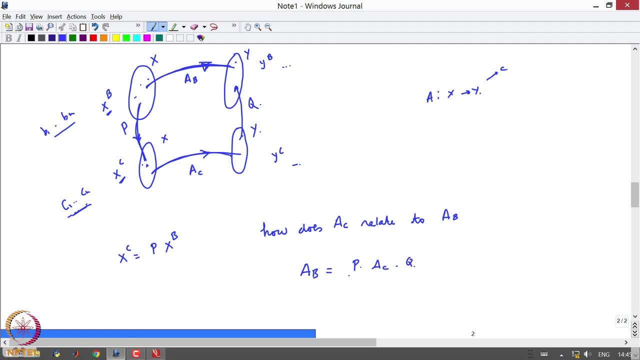 then jump from here to here. These are exactly the same. Now, a special case of this could be when- let me just take a different color- when x and y are the same. So in this case, x and y can be also can also be of different dimensions, So not need not necessarily be. 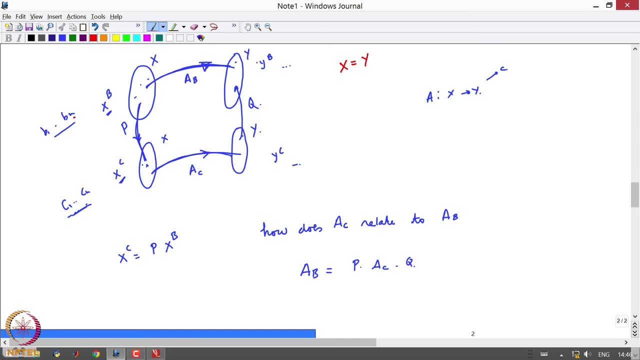 this is. this is an s here and n here. this can be a different number also. So if x equal to y, ok, So what will be this one? So this is, this is x. this is also x, with the similar changes over here. So if I can go from x B to x C via this matrix, P.